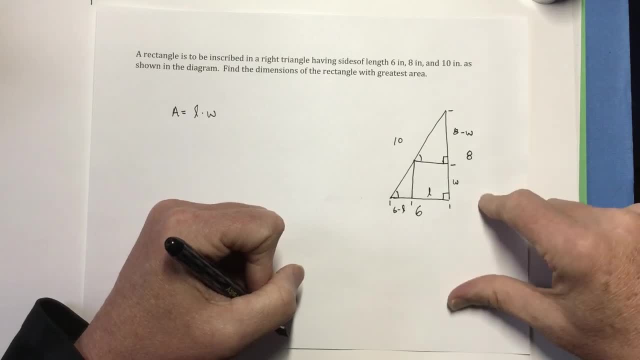 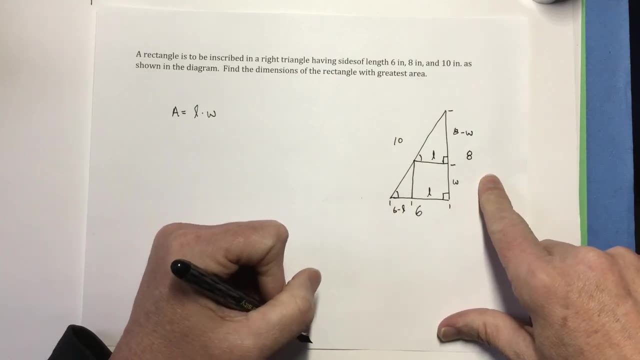 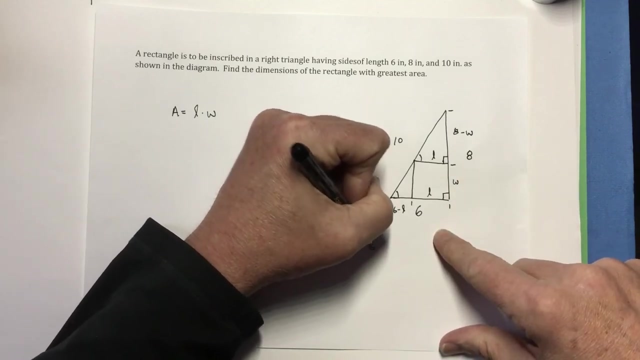 And that's 10.. All right, So what do I know? I know I'm going to label this L. It's the same thing. I know that L is to 6 as 8 minus W is to 8.. 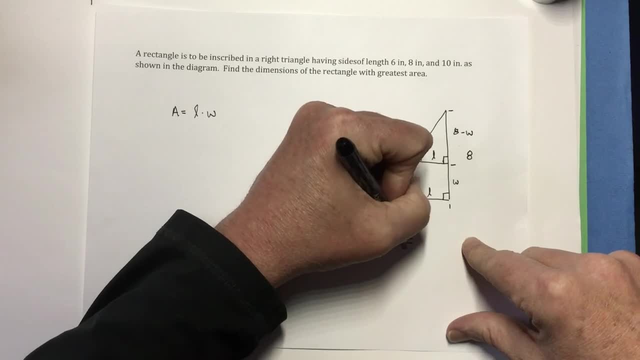 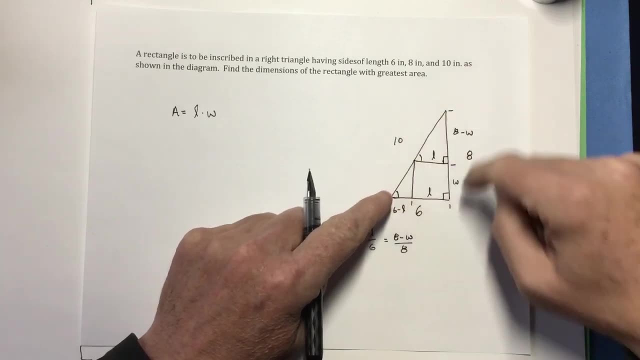 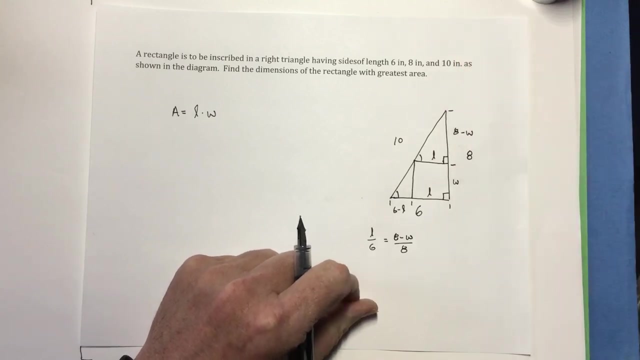 8 minus W is to 8.. In other words, this short side of this triangle, this triangle is to the short side of the large triangle, as the other leg of this triangle is to that leg of the large triangle. So there we go. 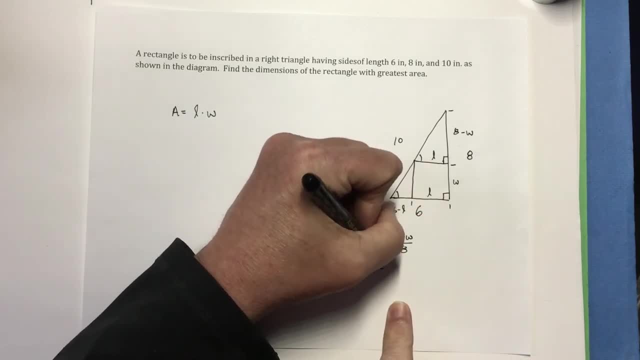 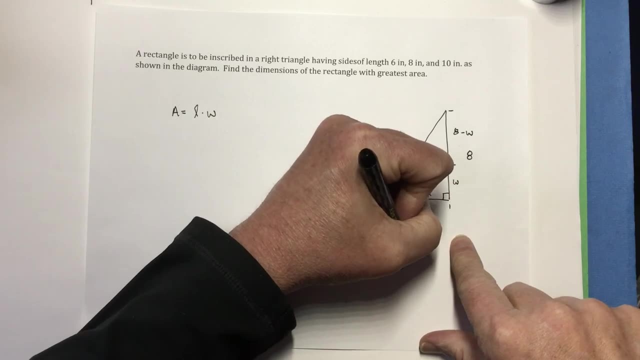 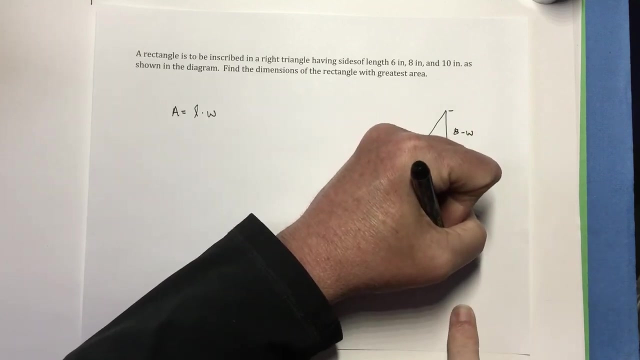 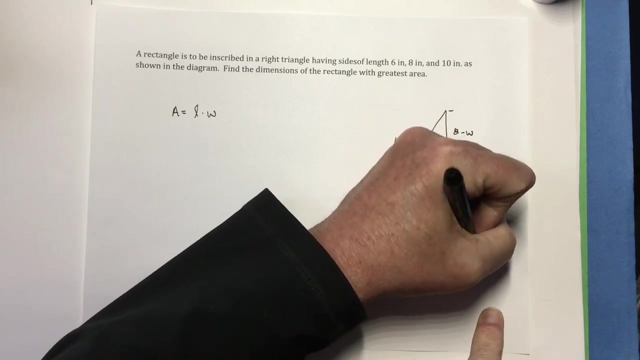 So I'm going to multiply by 6.. So I now have: L equals 6 times that, which is going to be 48 minus 6W over 8,, which will be 6 minus 6 over 8 is 3 fourths W. 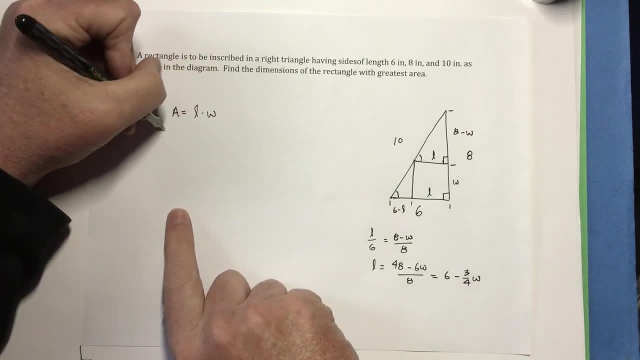 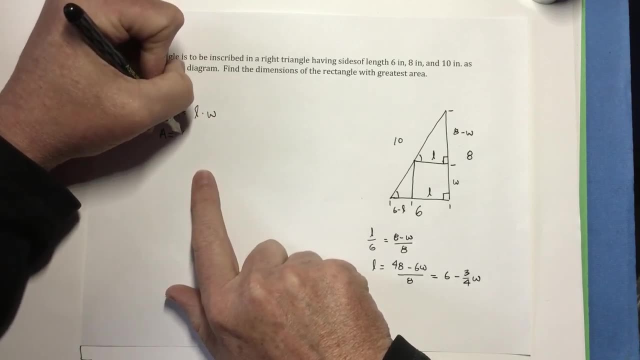 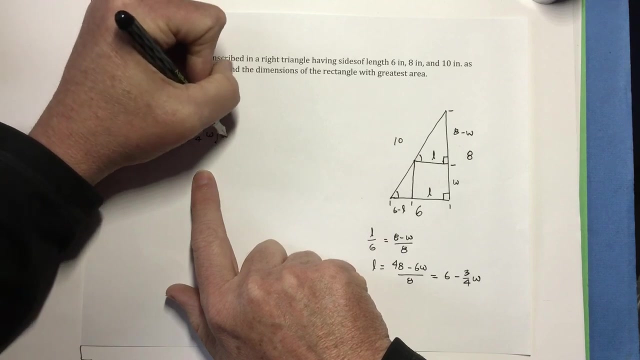 Okay, Good. So now that means I can rewrite my area in just terms of W. So if L is 6 minus 3 fourths W, then I can say the area I'm interested in is 6 minus 3 fourths W times W, All right. 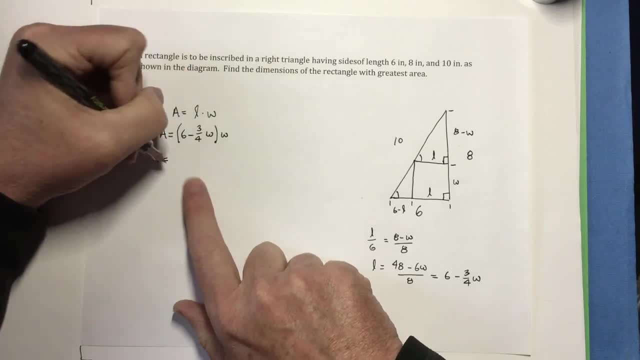 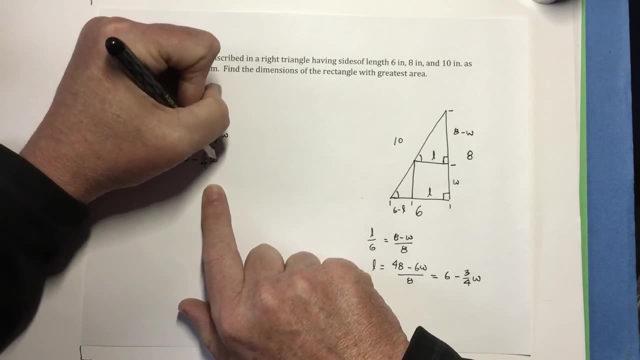 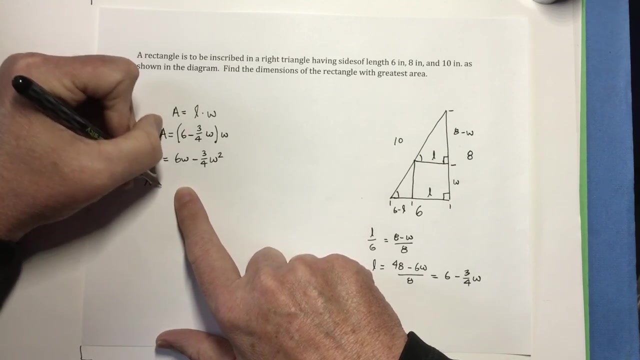 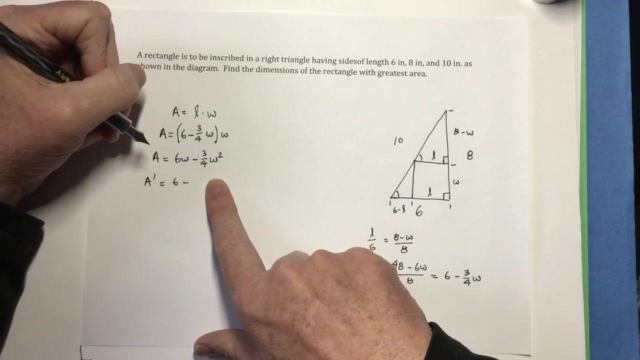 Which means area. So the area I'm interested in is 6 minus 3 fourths W times 3 fourths W times 3 fourths W. Okay, Splendid, I will now take the derivative of the area. A prime is going to be 6 minus 2 times 3 fourths W, which is 3 halves W. 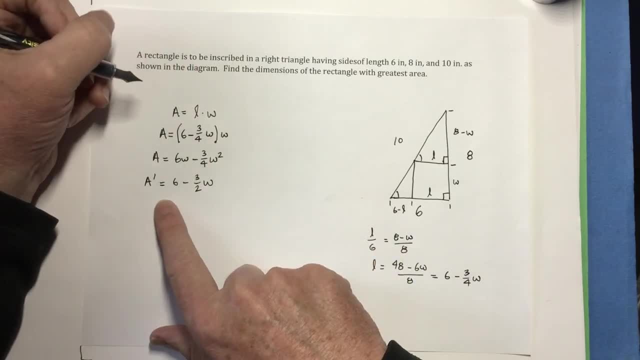 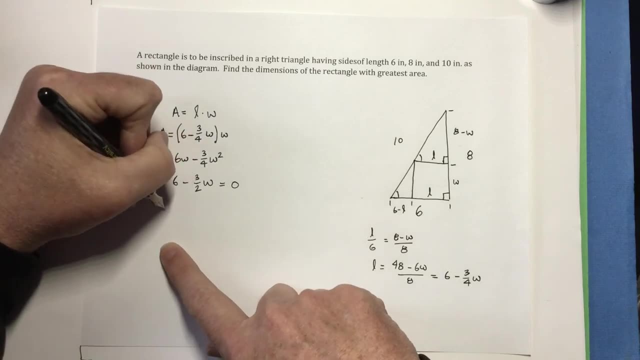 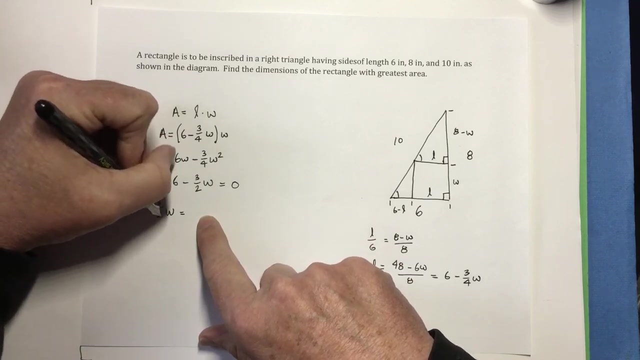 Okay, And now to maximize that, I want to findset it equal to 0. So let's do that. If I set this equal to 0, that means W equalswell, let's dolet's skip a step here. 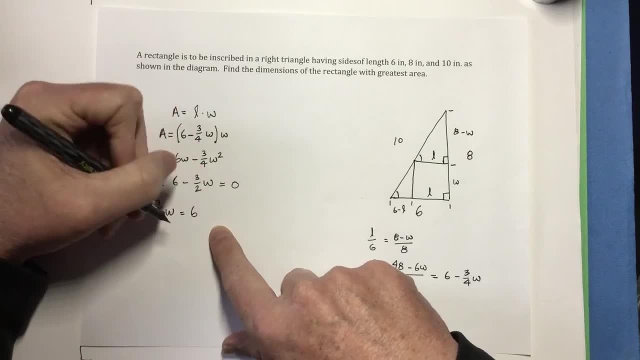 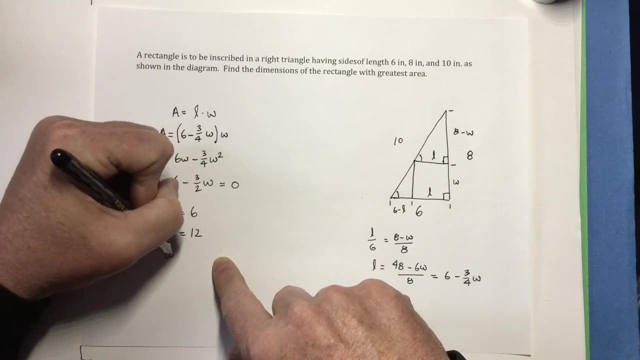 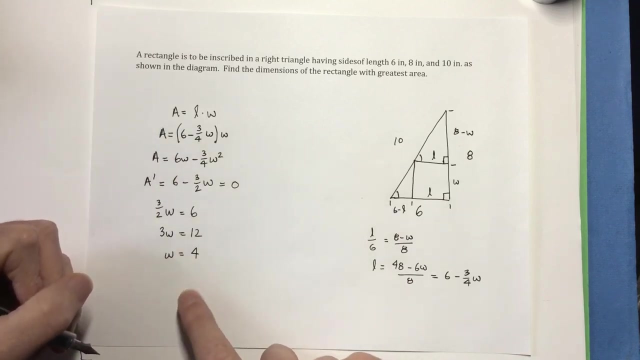 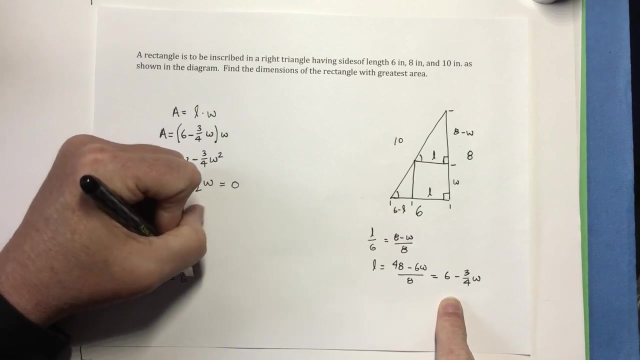 3 halves W will equal 6.. So 3W equals 2 times 6,, which is 12.. So W equals 4.. Okay, Splendid, All right, Splendid. Now, if W equals 4,, then I know that L equals 6 minus 3 fourths times W, which is 4.. 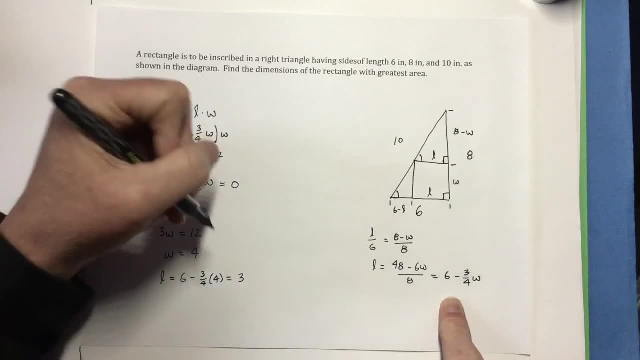 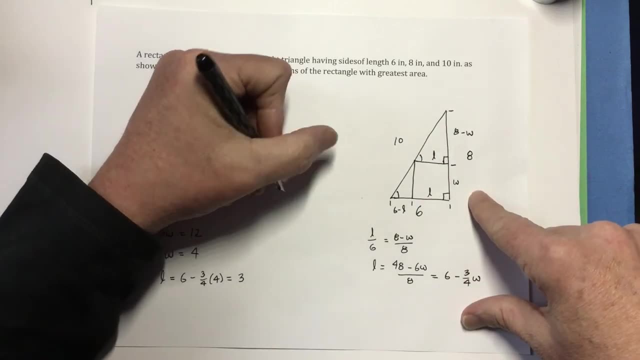 The fourths cancel out. It's 6 minus 3, which is 3.. So the dimensions of the greatest area that can be inscribed in there will be the situation where W is 4 and L is 3.. Okay, 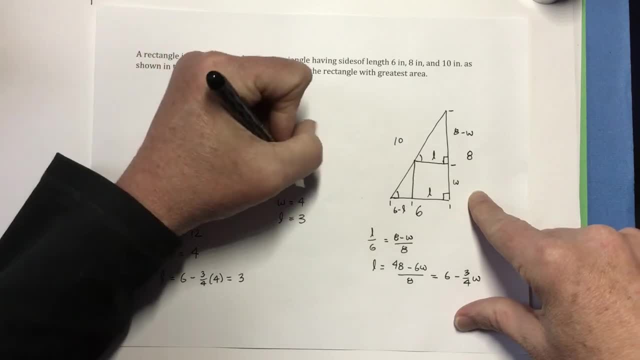 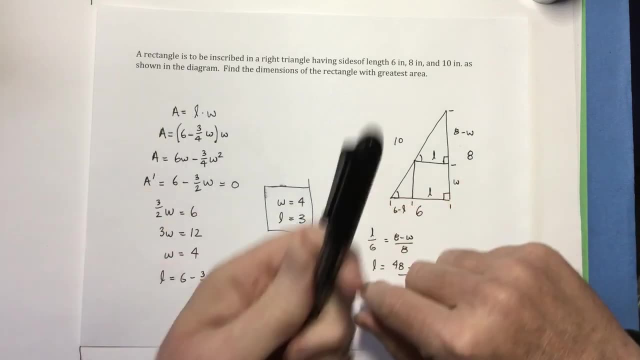 All right, Let's do that again. So W equals 4.. L is 3.. Well, there you go. I do not recommend you do your math in pen, but I wanted this to show up better on the video. And you see, that's what happens right there. 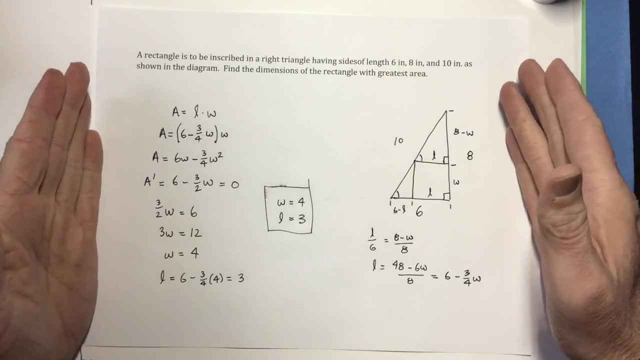 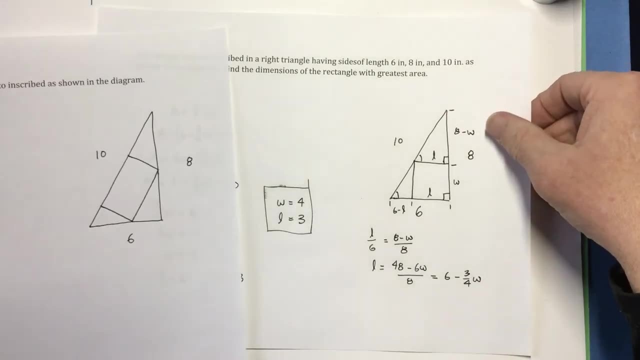 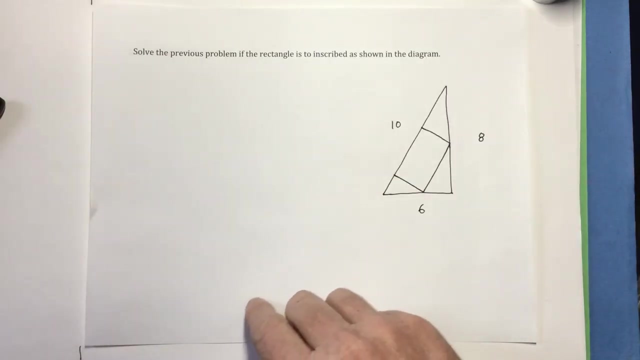 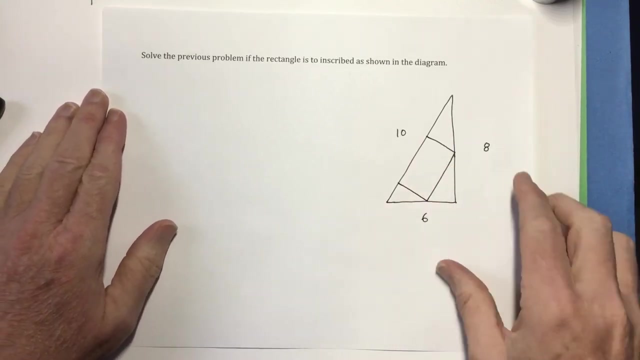 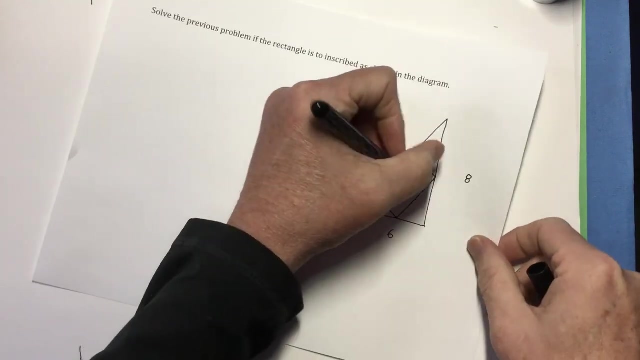 See that smudge? Oh Okay, So there you go, There's that one. Now the companion problem to this is the same problem, but in this case theyou. the rectangle to be maximized is situated this way in my inscribed, in my triangle. so again, i'm going to call this length here. 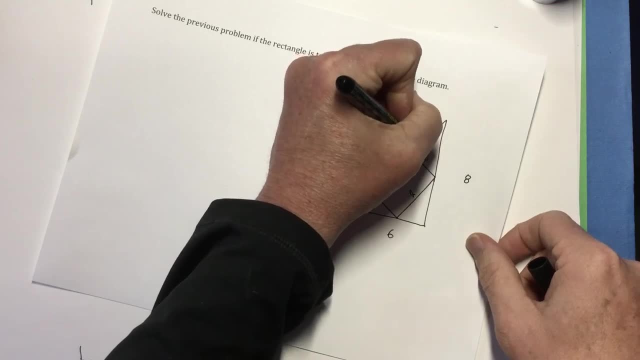 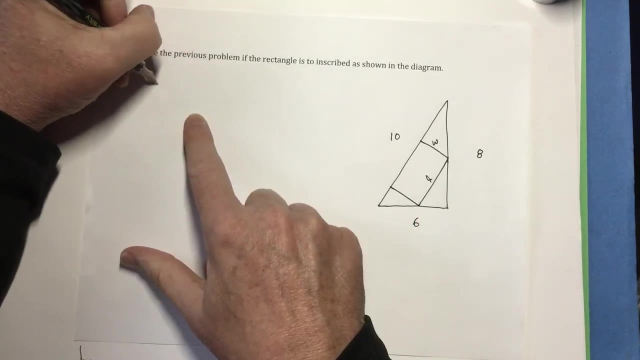 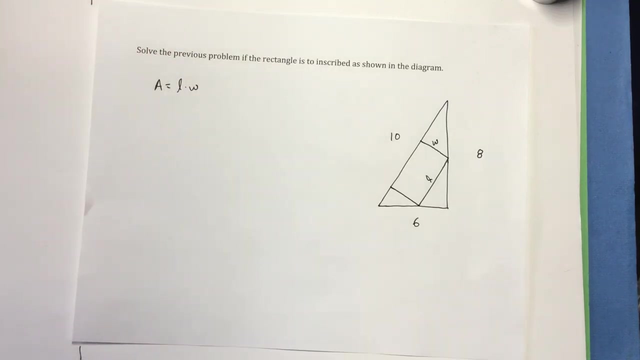 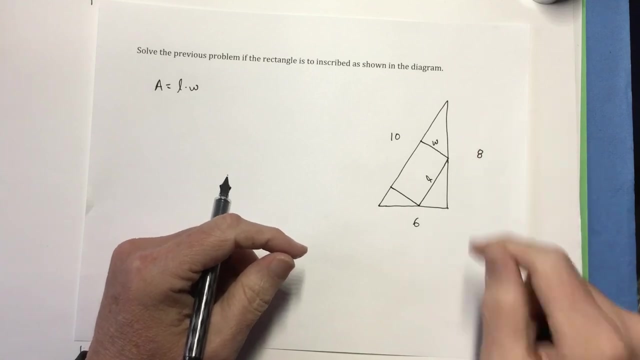 i call this width all right, so my area that i'm trying to maximize will simply be length times width, all right. so now, what do we have here? well, again, it's the same idea. we've got similar triangles all around, so that triangle is similar to the large one. 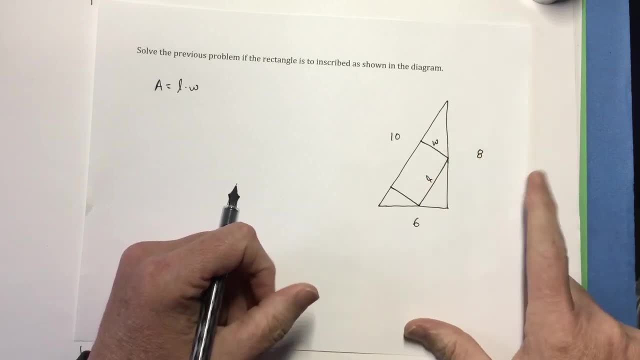 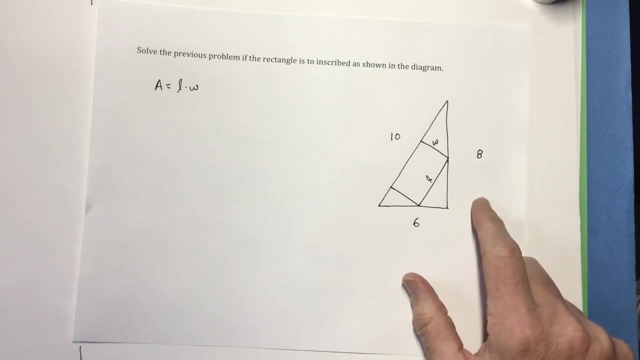 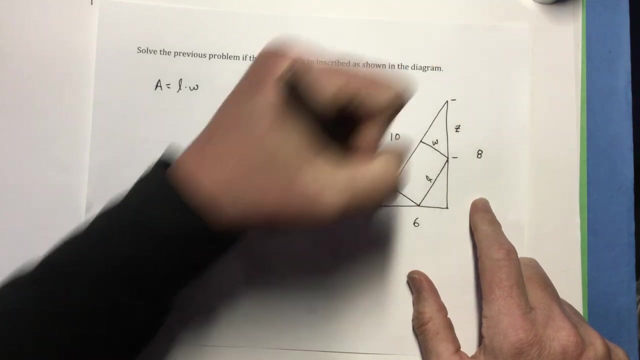 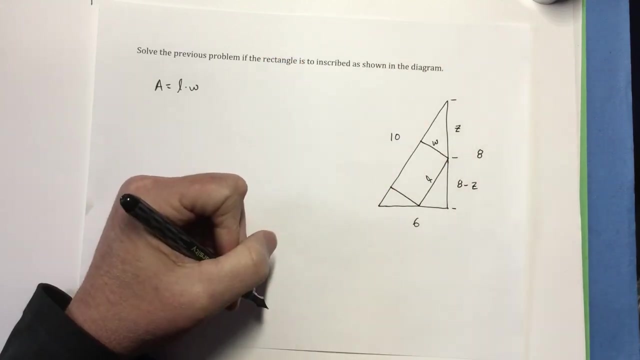 which is similar to that, one which is similar to that. so let's see, okay, i'm going to need something else here, so i will use the letter z. i'm going to label this distance right here: z. that means this distance here would be 8 minus z. all right, so what does that tell me? well, that means that. 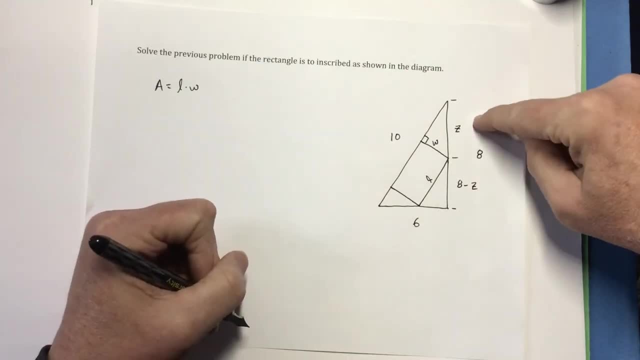 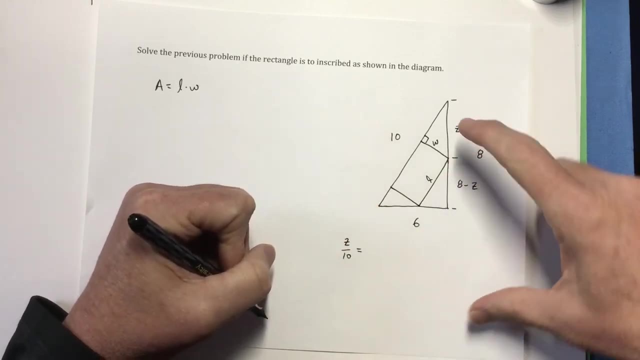 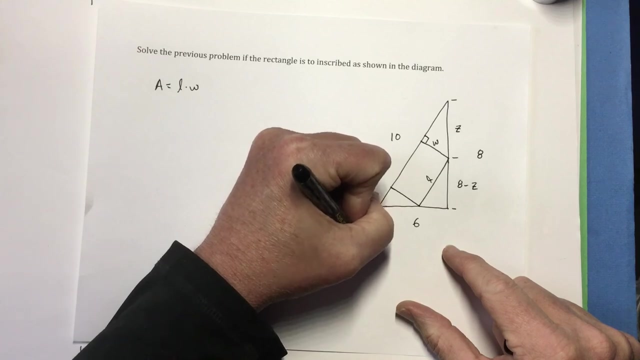 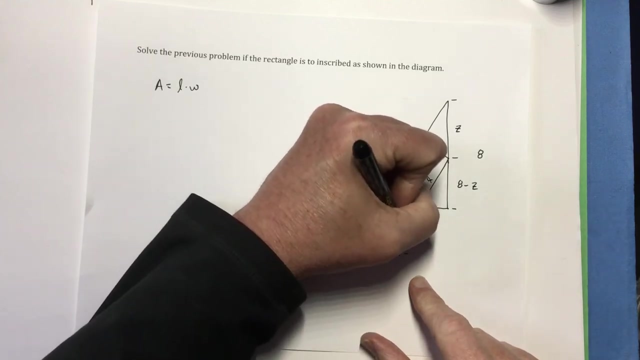 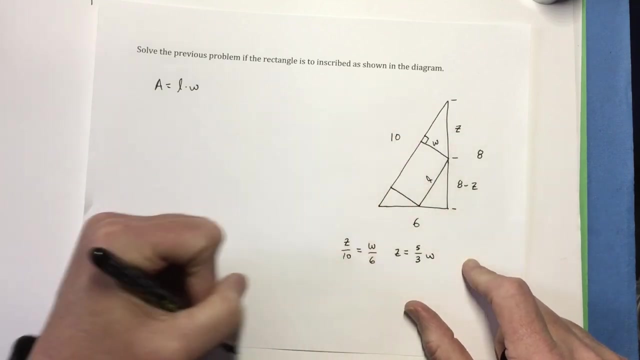 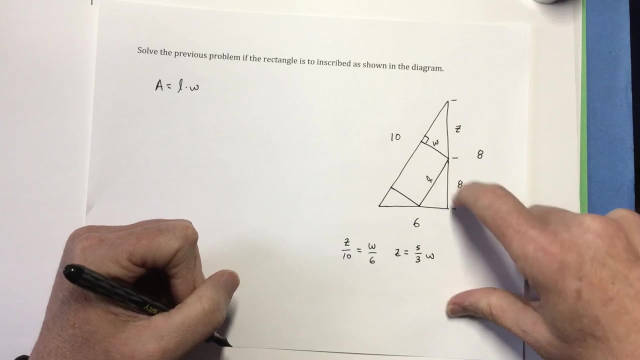 this is our right angle right here- that z is to 10, z is to 10 as w is to 6. excellent, which means i can write that, as z equals 10, w over 6, which is thirds w. okay, now what else do i know? i know that if i look at this triangle right here. 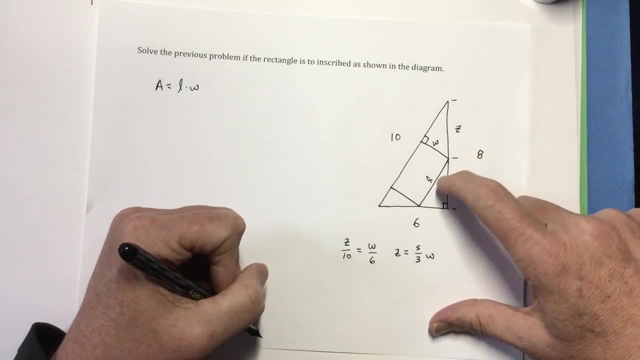 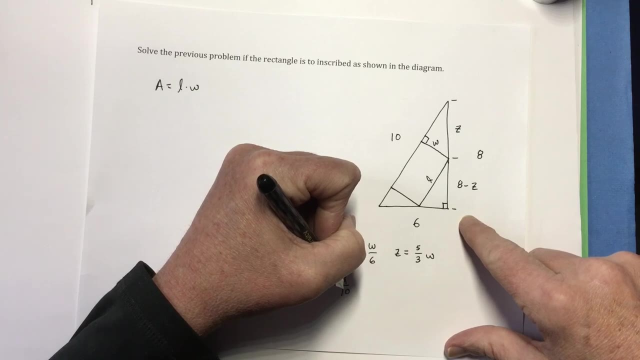 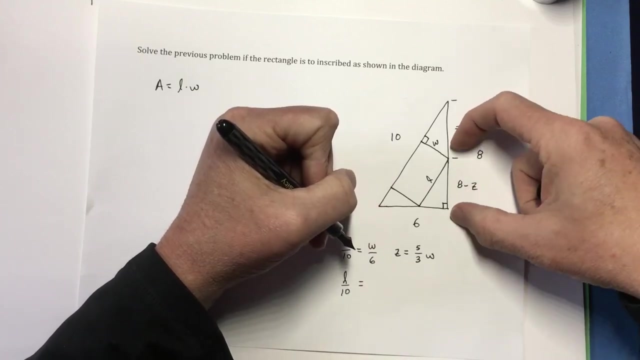 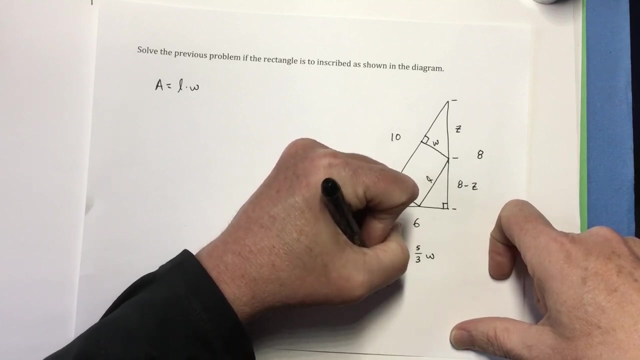 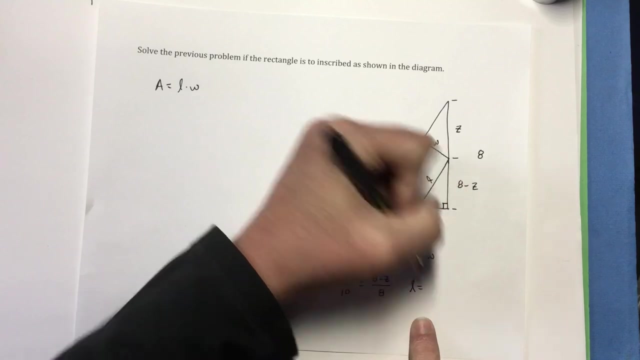 that, let's see l, our length is to 10, as let's see. well, yeah, um, and that side then is to the entire side. so l is to 10, as 8 minus z is to 8. so i'm going to multiply by 10. that means l equals. 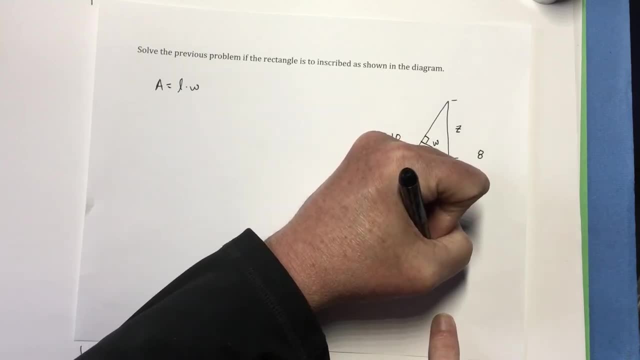 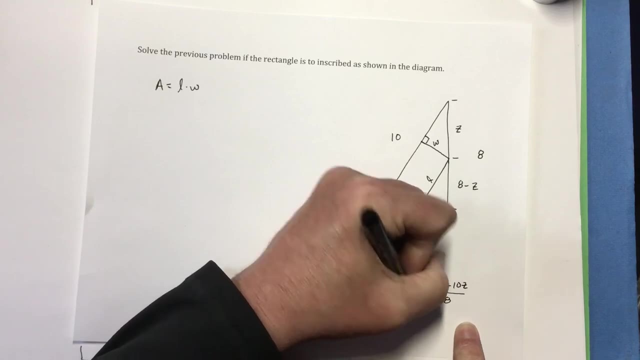 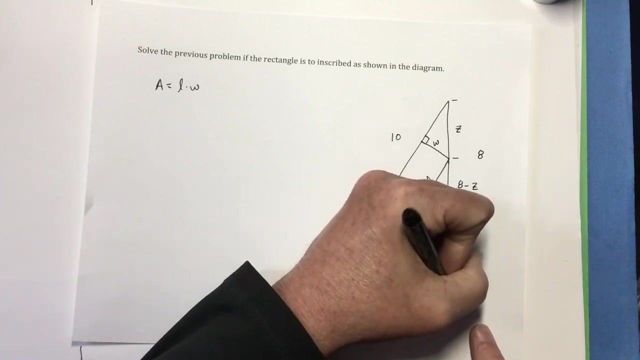 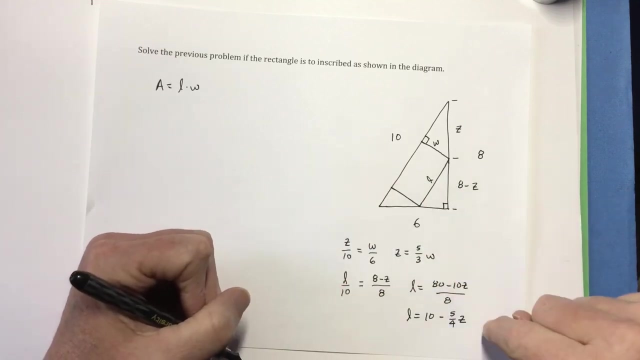 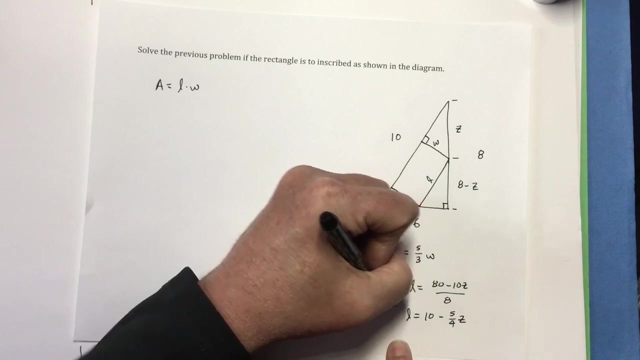 uh, 10, 80 minus 10 z over 8, which means l equals 10 minus. i can reduce that to five force, five force z. okay, now i know that z equals five thirds w, so i can further take this l right here i'm gonna. 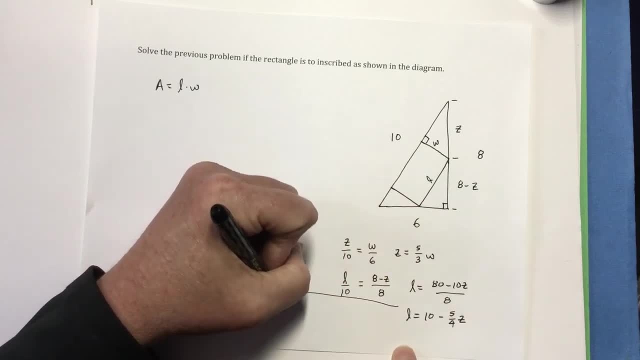 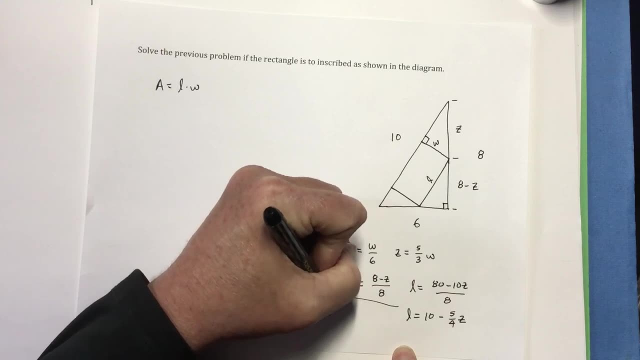 have to bring it clear over here because i didn't plan too well. so l is going to be equal to 10 minus 5 force times z, which is 5, 3 w. so that means l finally is 10 minus 25, 12 w. 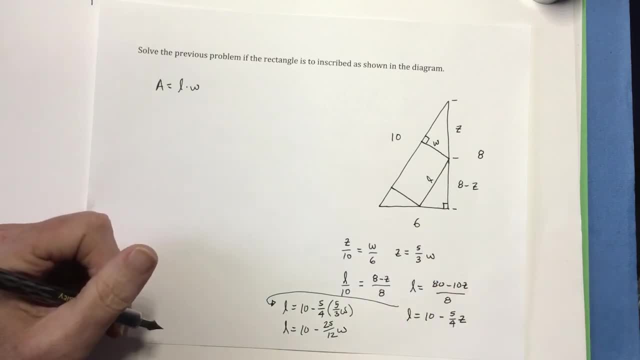 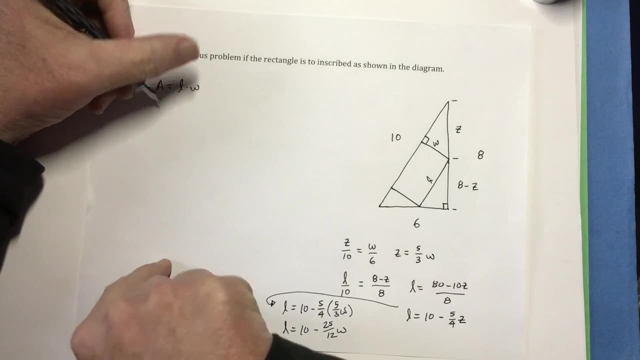 yeesh, could have written that a little better, i think, but i'm not going to fix it. so there's my l. so now i can use that in here and reduce my function to just one variable. so that means my new area function will be l, which is 10 minus.